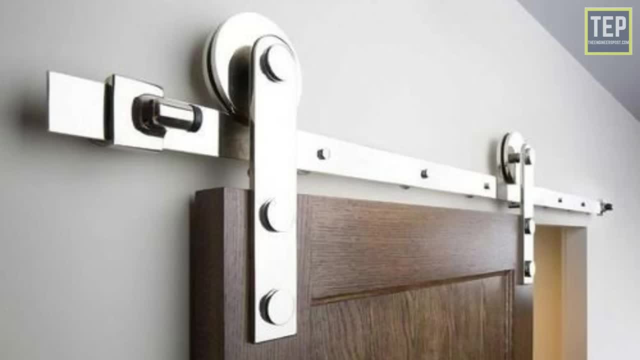 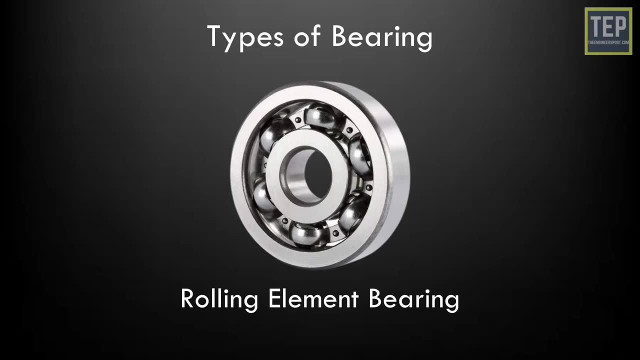 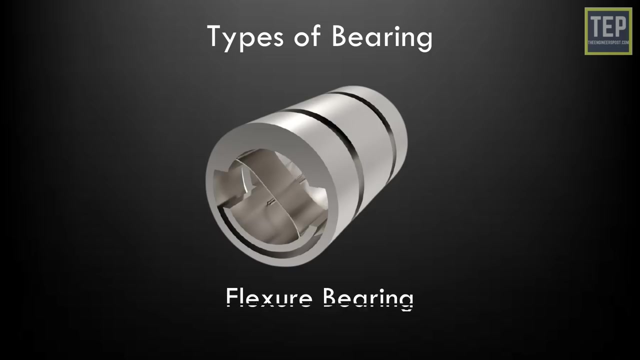 friction is reduced, speed and efficiency of an object will be enhanced. Different types of bearings are used for various applications, such as rolling, element bearing, plane bearing, fluid bearing, magnetic bearing, joule bearing and flexure bearing. But first let we know about what is the purpose of bearings. 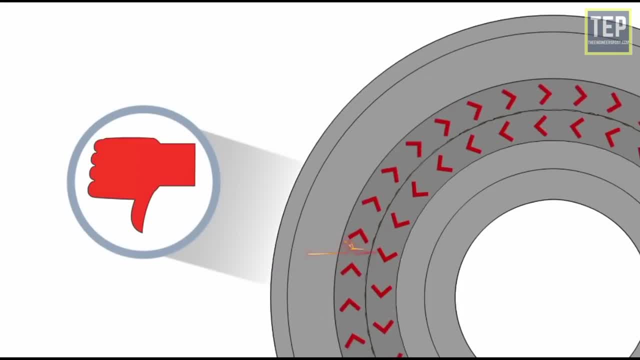 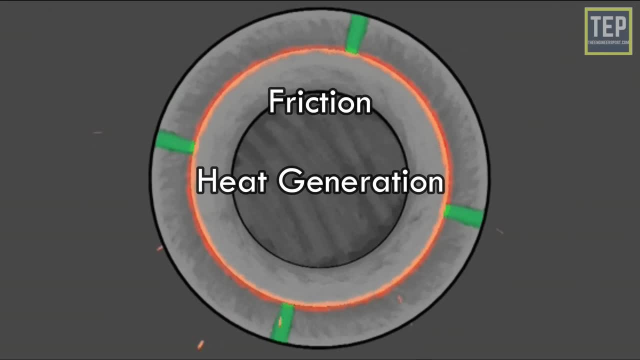 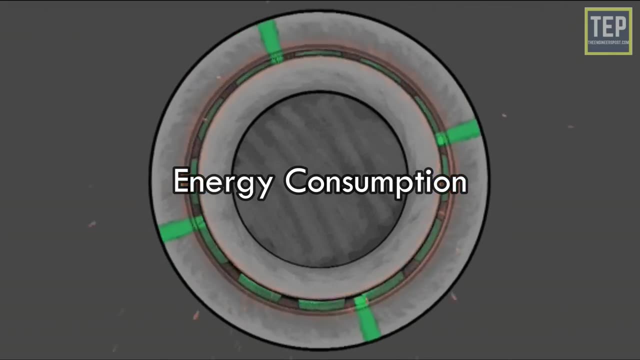 The main purpose of bearings is to prevent direct metal-to-metal contact between two elements that are in relative motion. This prevents friction, heat generation and, ultimately, the wear and tear of parts. It also reduces energy consumption, as sliding motion is replaced with low friction. 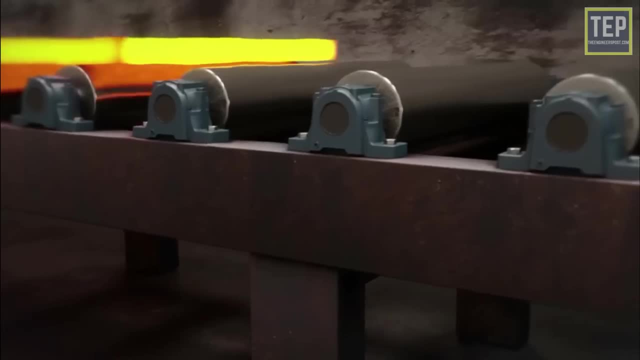 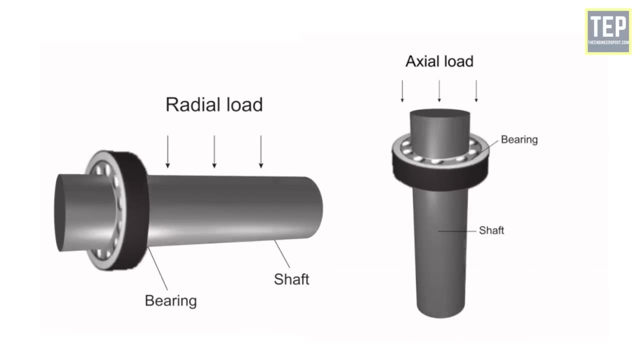 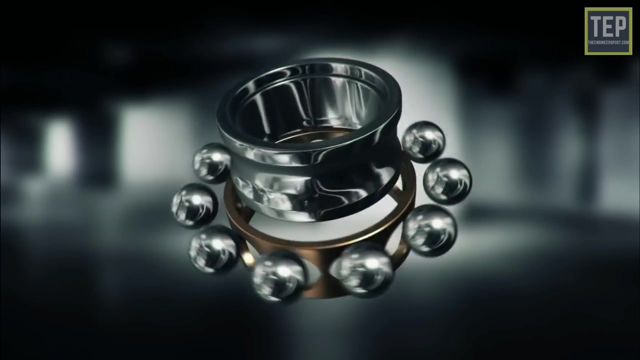 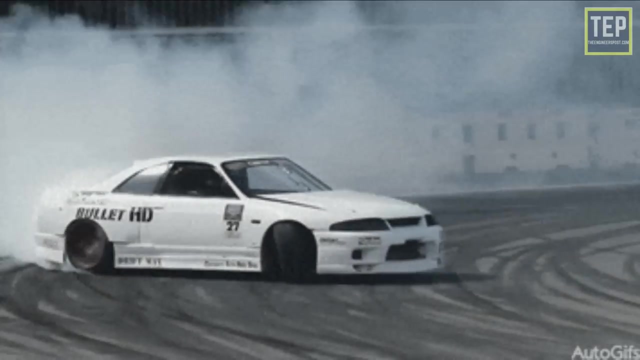 rolling. They also transmit the load of the rotating element to the housing. This load may be radial, It may be axial or a combination of both. Rolling element bearings contain rolling elements in the shape of balls or cylinders. We know that it is easier to roll a wheel than slide it on the ground, as the magnitude of 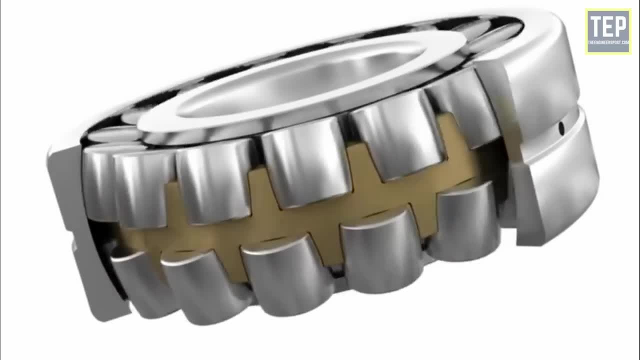 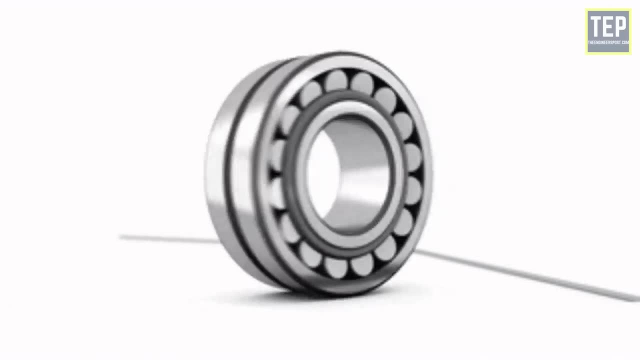 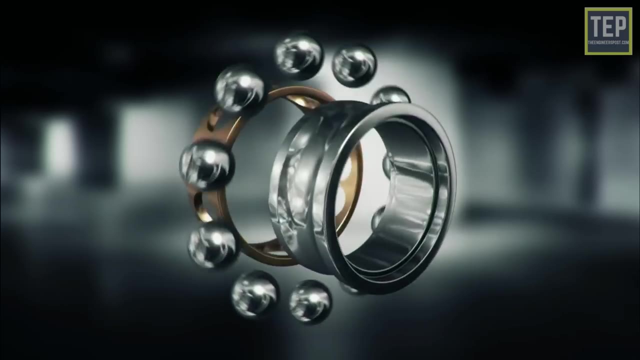 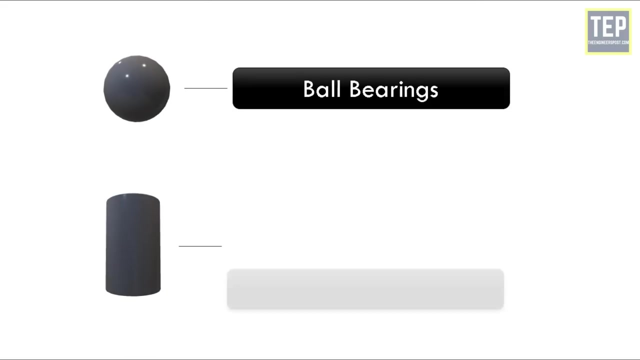 rolling friction is lower than sliding friction. The same principle is in work here. These bearings are used to facilitate the free movement of parts in rotational motion. Rolling elements carry the load without much friction, as the sliding friction is replaced with rolling friction. Rolling element bearings can be subdivided into two major types: ball bearings and roller bearings. 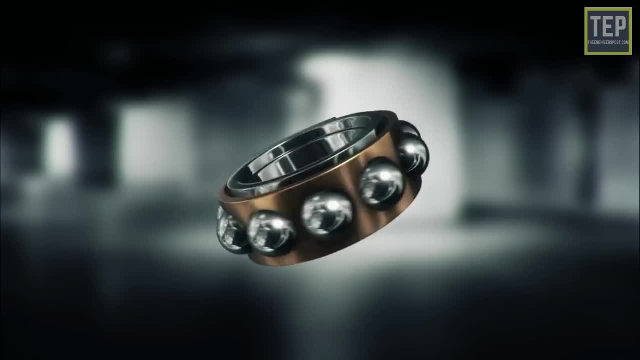 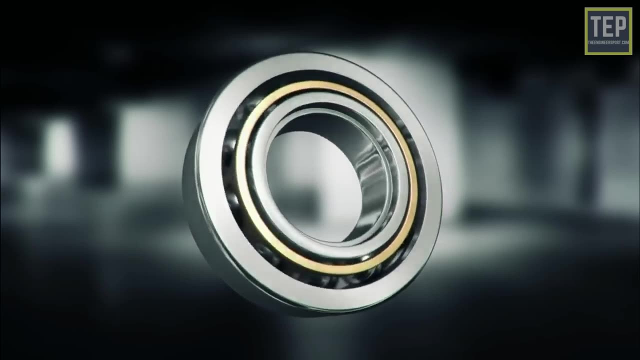 Ball bearings are one of the most common types of bearing. It consists of a row of balls. as rolling elements. They are trapped between two annulus-shaped metal pieces. These metal pieces are known as races. These metal pieces are called races. The inner race is frayed and the inner race 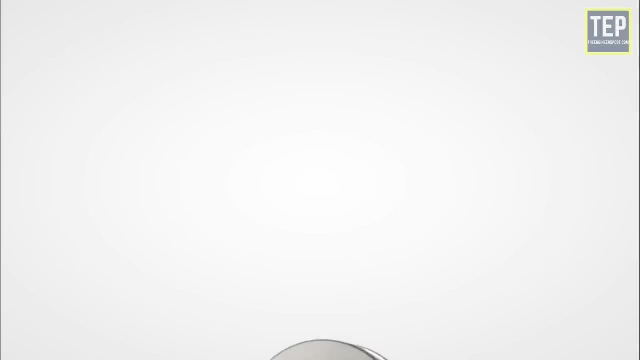 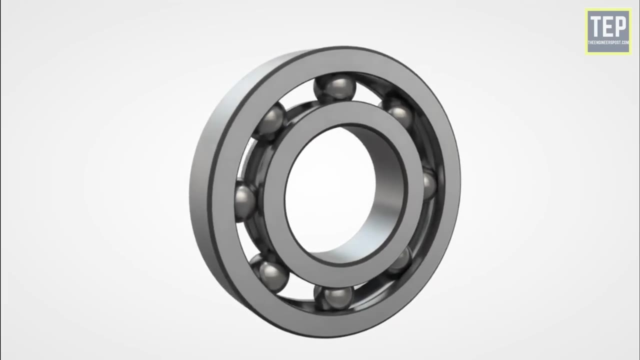 is frayed. In this case, the inner race is frayed. The inner race is frayed and the inner race is to rotate, while the outer race is stationary. Ball bearings provide very low friction during rolling but have limited load carrying capacity. This is because of the small area of contact. 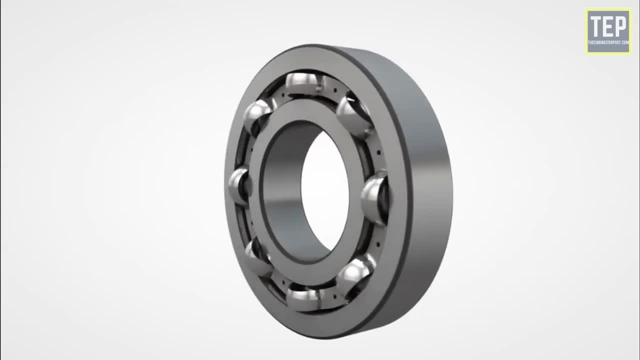 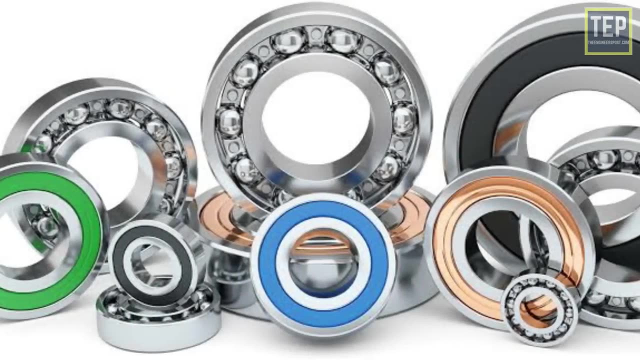 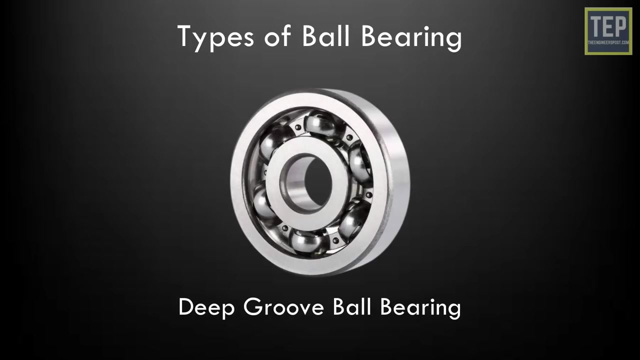 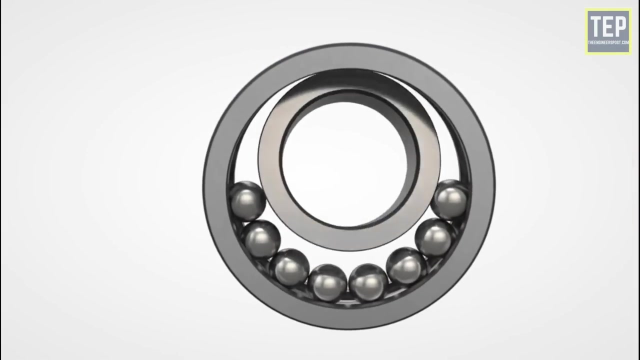 between the balls and the races. They can support axial loads in two directions, besides radial loads. Depending on the application, different types of ball bearings are available to choose, such as deep groove ball bearings. This is the most widely used ball bearings. Trapped between the two races is a ring of balls that transmit the load and allows rotational. 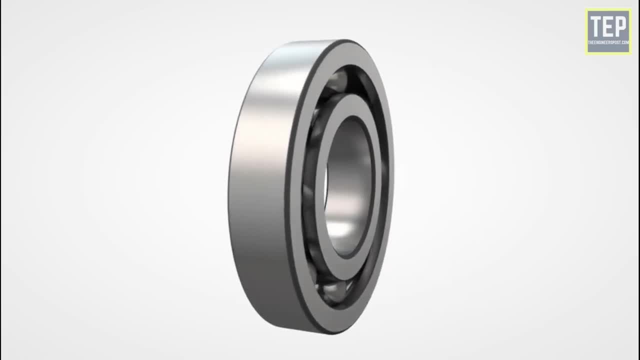 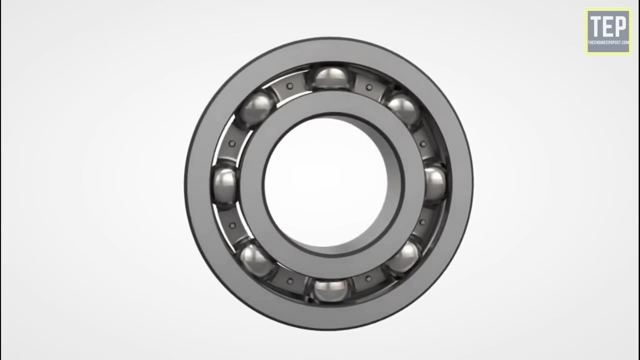 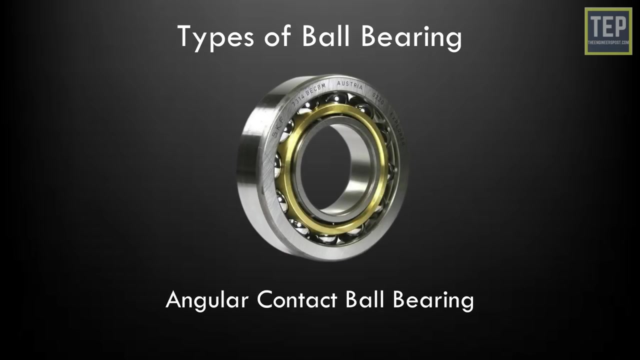 motion between the two races. The balls are held in place by a retainer. They have very low rolling friction and are optimized for low noise and low vibration. Angular contact Ball bearings In this ball bearing the inner and outer races are displaced with respect to 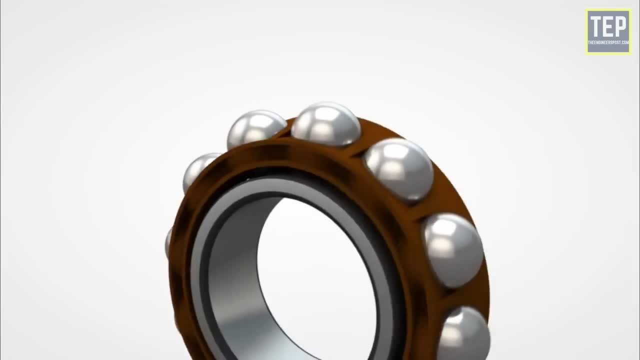 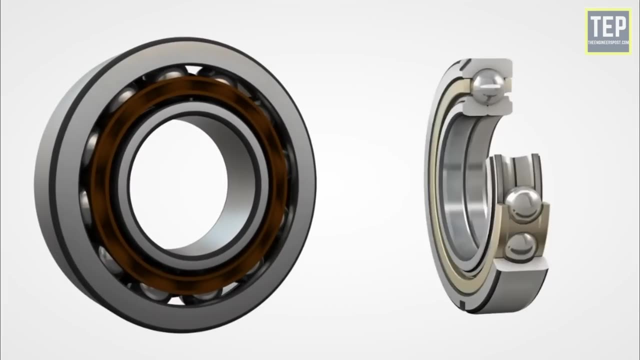 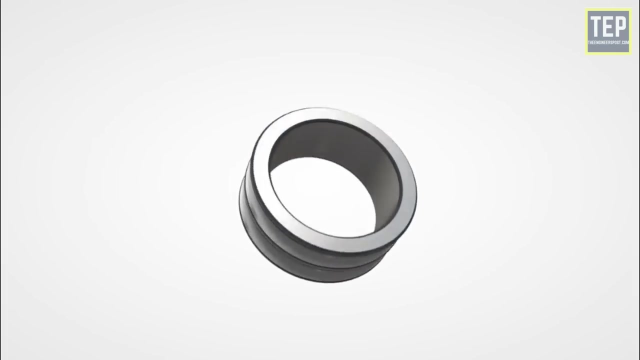 each other along the bearing axis. This type is designed to handle greater amounts of axial loads in both directions, in addition to radial loads. Self-aligning Ball bearings. This type of ball bearing The inner ring has deep grooves similar to deep groove ball bearings, followed by two rows of. 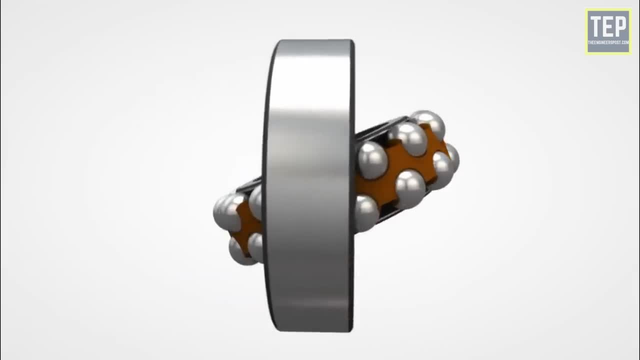 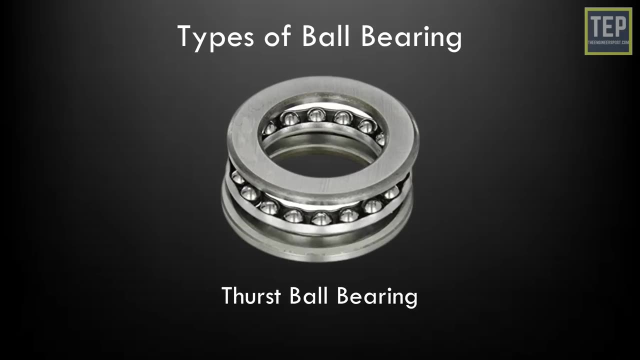 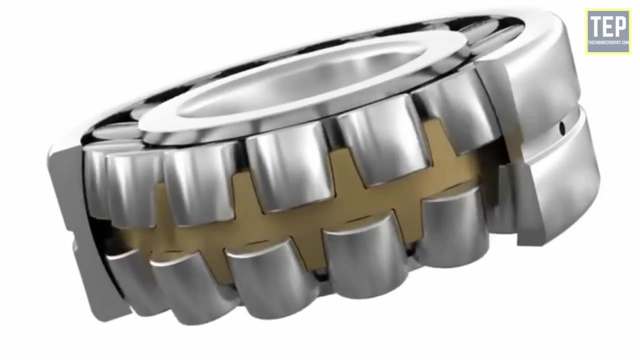 same peroxide, Türmungs, amputations and the other ring. The outer ring has a concave shape and this grants the inner ring на. These bearings exhibit low noise, smooth operation and are capable of high-speed applications. Roller bearings maintain accurate alignment of every part over a long period of time and can carry. 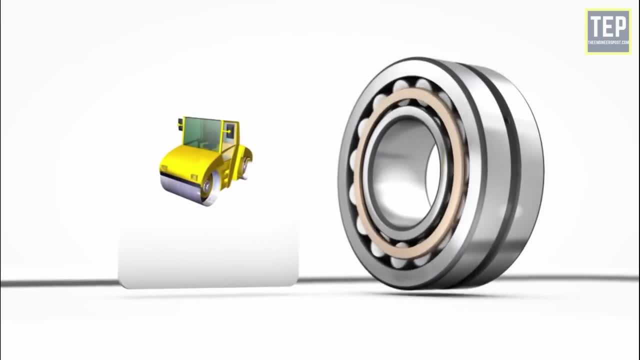 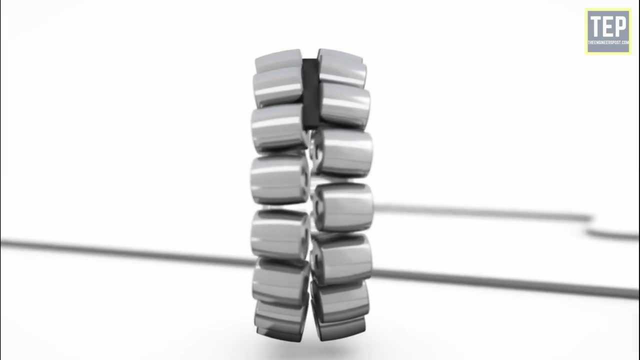 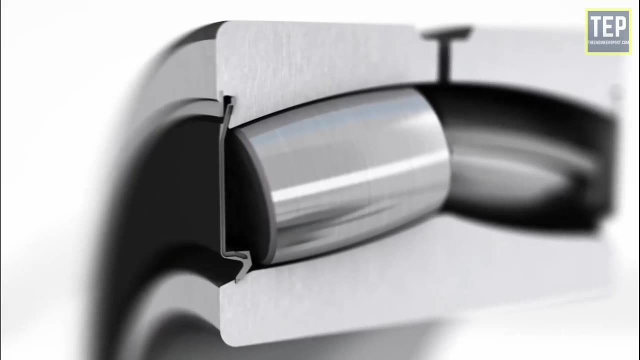 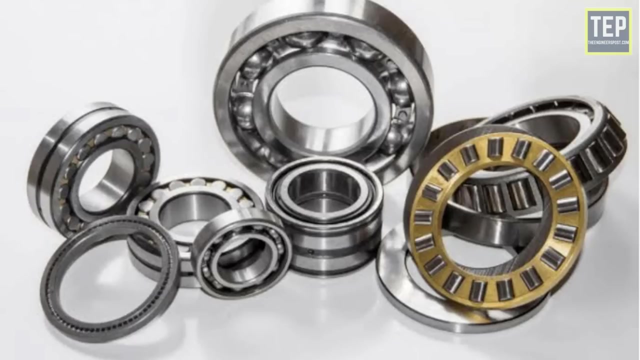 heavy momentary load. this renders them suitable for machinery which requires to frequent start and stops. rolling makes the line contact with their races, while balls make point contact. it has a higher load carrying capacity. roller bearings contain cylindrical rolling elements instead of balls as load carrying between the races in roller bearings. there are also various 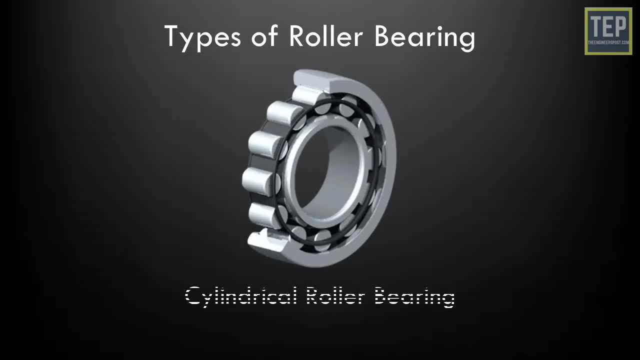 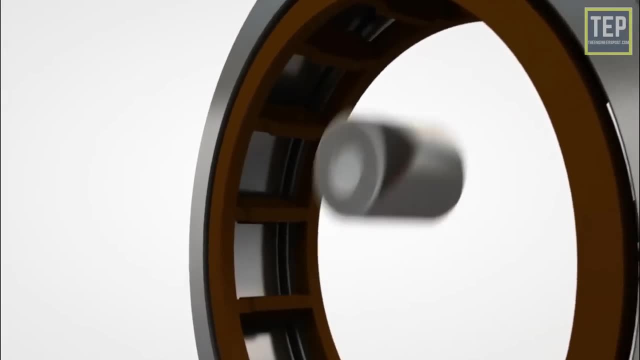 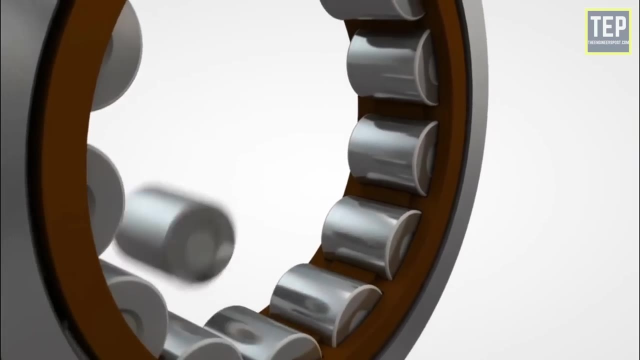 types such as cylindrical roller bearings use line contact between the rolling elements and the raceways, which optimizes the distribution of stress factors at the point of contact. this cylindrical roller bearings have a very high radial load rating. depending on the design, they may also be able to transmit a limited amounts of axial loads. 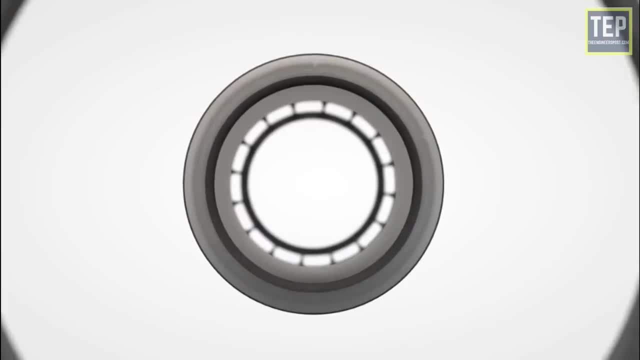 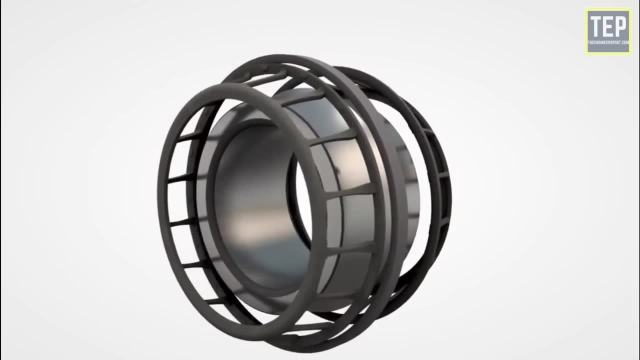 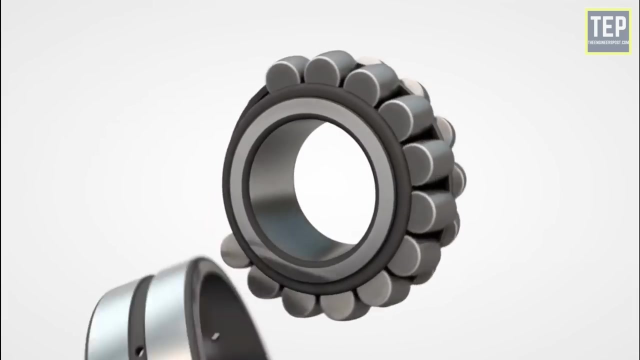 spherical roller bearings. these bearings are very robust and work on the same principle as self-lining bearings, with the exception that they use spherical rollers instead of ball rollers, allowing higher loads to be supported. spherical roller bearings are suitable for absorbing high radial loads and moderate axial loads. 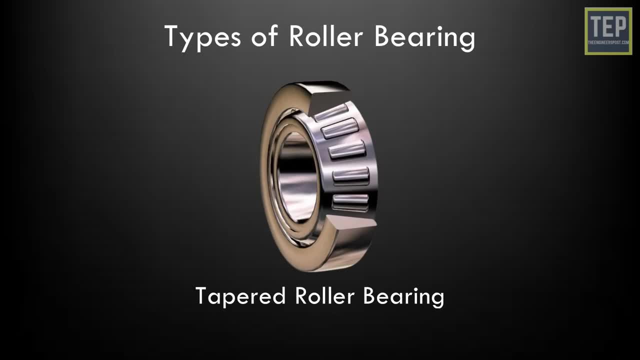 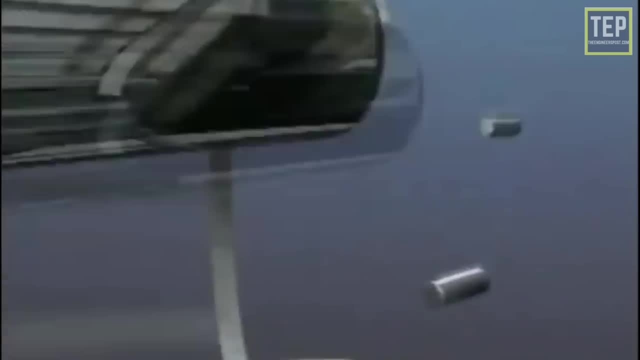 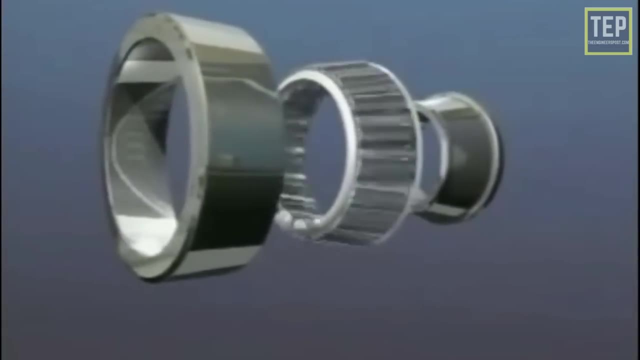 the tapered roller bearings contain sections of a cone as a load carrying element. these rollers fit between the two races that are also sections of a hollow cone. if the races and the axes of rollers were extended, they would all meet at a common point: tapered roller bearings are designed to handle higher axial loads besides radial loads. 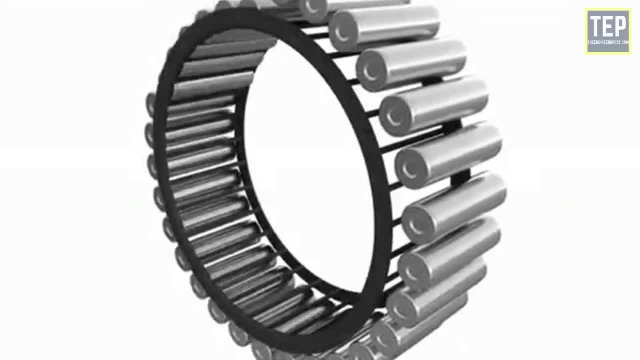 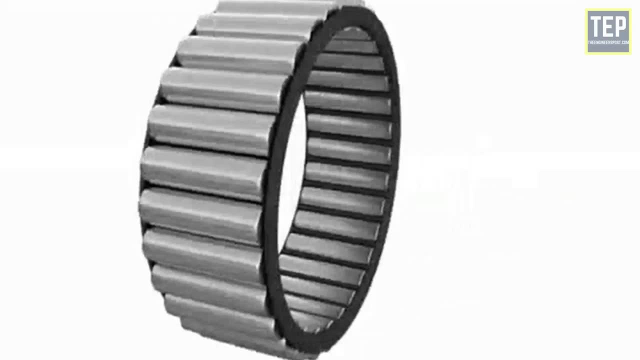 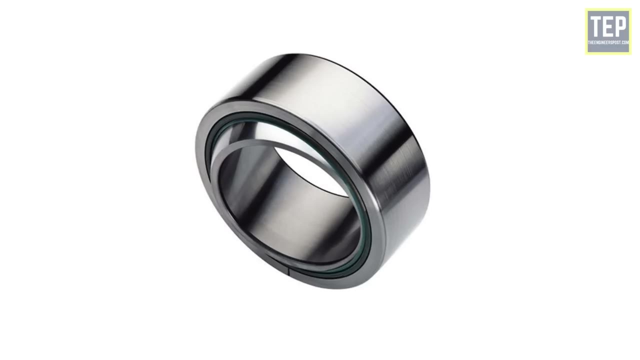 needle roller bearings are a special type of cylindrical roller bearings which contain long, thin rolling elements. needle roller bearings have a high load rating and are only suitable for radial forces. the diameter of the roller bearing is the same as the diameter of a cylinder and the diameter of the roller is the same as the diameter of a cylinder. 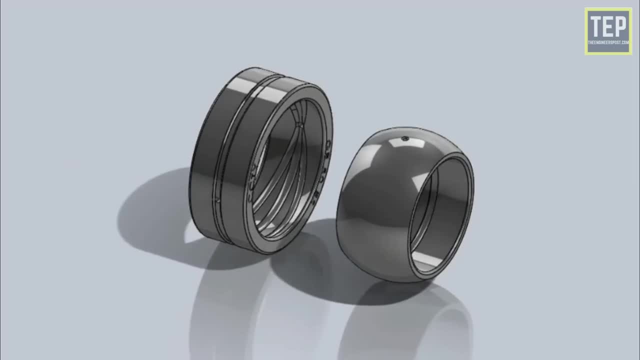 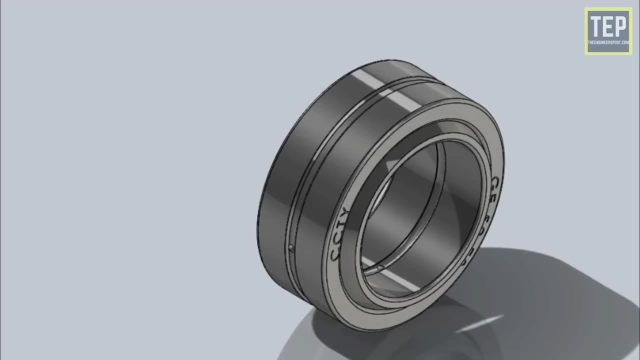 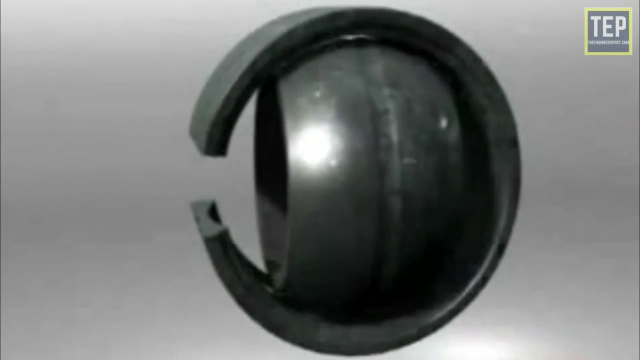 a plane bearing is the simplest type of bearing. it usually only consists of a bearing surface. there are no rolling elements. plane bearings are used for rotational, sliding, reciprocating or oscillatory motion. the bearing remains fixed while the journal slides on the bearing's inner surface. the bearing is basically a sleeve mounted on the shaft and fit into the bore. plain bearings are. 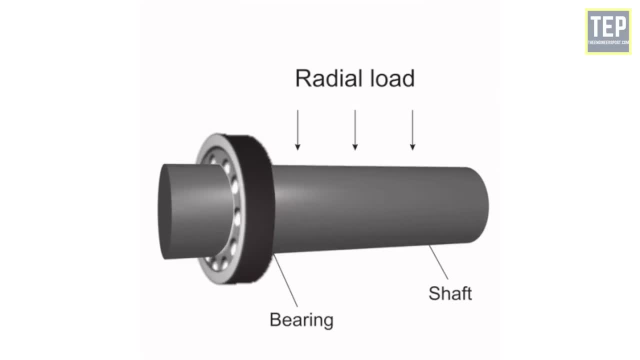 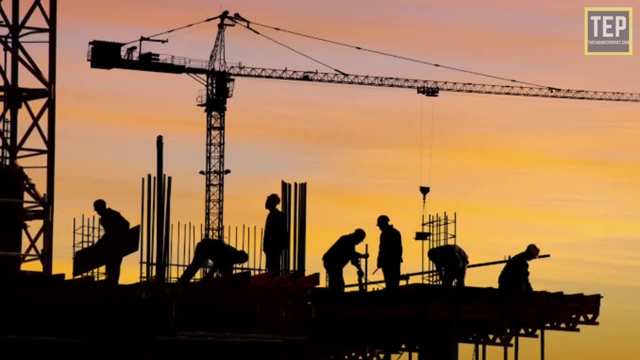 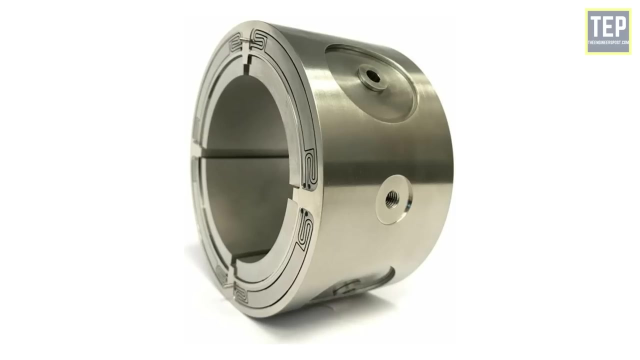 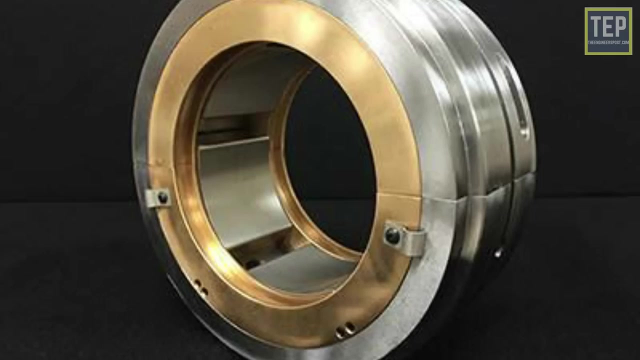 inexpensive, compact and lightweight, high load carrying capacity. it is used extensively in applications in the agriculture, automotive, marine and construction industry. fluid bearing is a special type of bearing that relies on pressurized gas or liquid to carry the load and eliminate friction. these are used to replace metallic bearings where 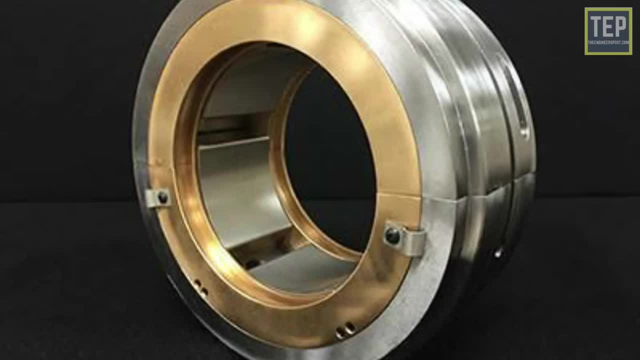 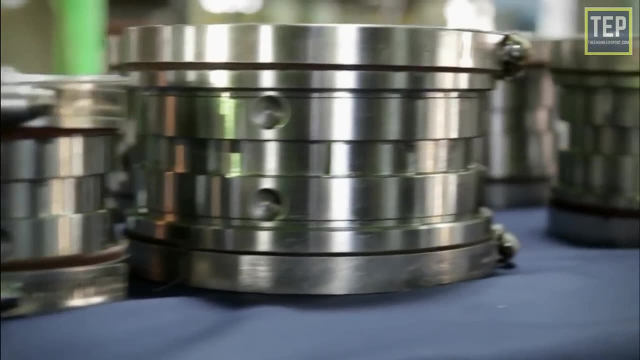 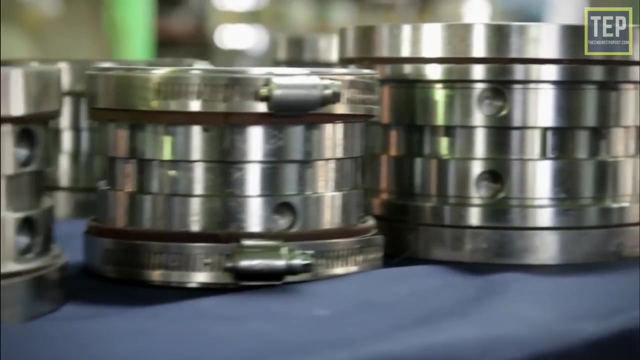 they would have a short life. in addition to high noise and vibration levels, these bearings are used in machines that work at high speeds and loads. while the initial costs are higher, the longer lifespan in tough conditions makes up for it to run longer time. magnetic bearings use the concept of magnetic. 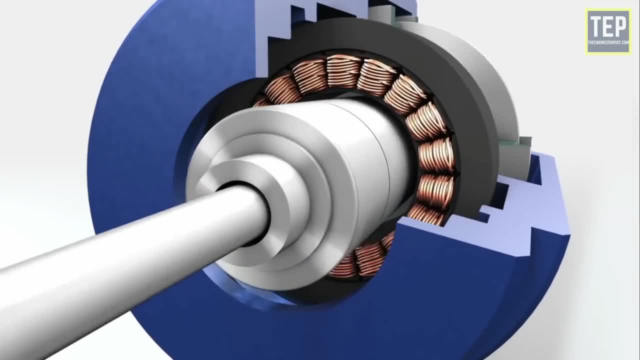 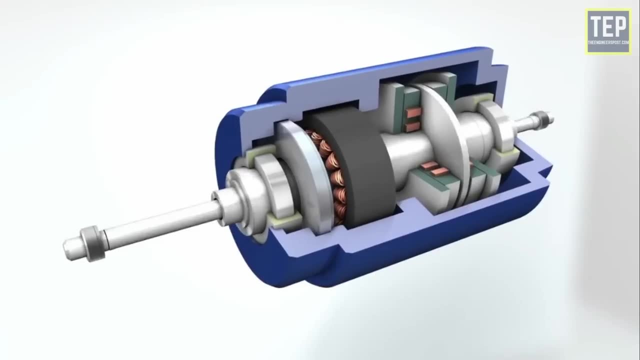 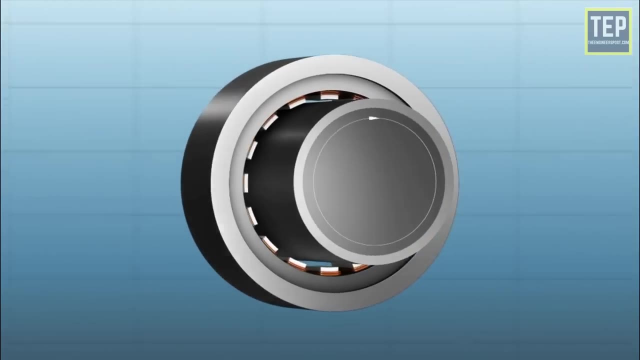 levitation to hold the shaft midair. as there is no physical contact, magnetic bearings are zero wear bearings. there is also no limitation on the maximum amount of relative speed which it can handle. magnetic bearings can also accommodate some irregularities in shaft design, as the shafts position is automatically adjusted based on its